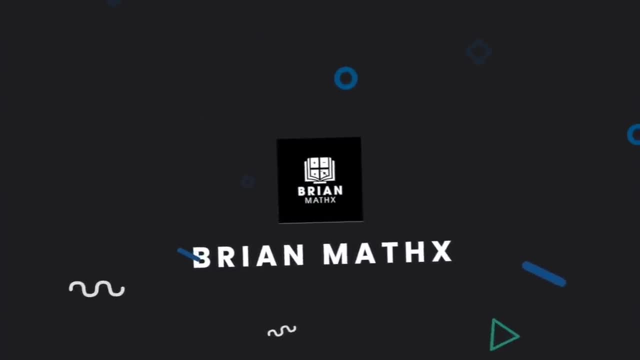 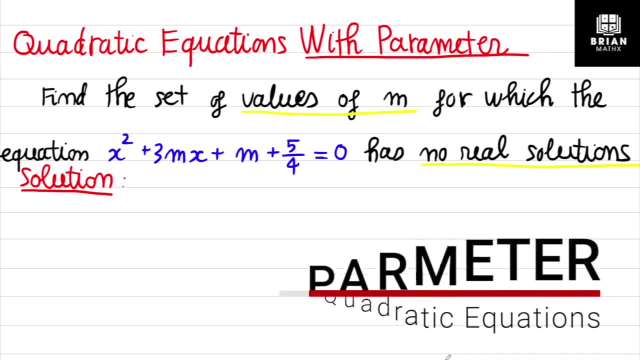 Hello guys, welcome back to my channel. In this video we continue learning about quadratic equation with parameter And for this question we have a very difficult question about the quadratic. You got the parameter in the equation, blue pen and you have to find the set of value of m. 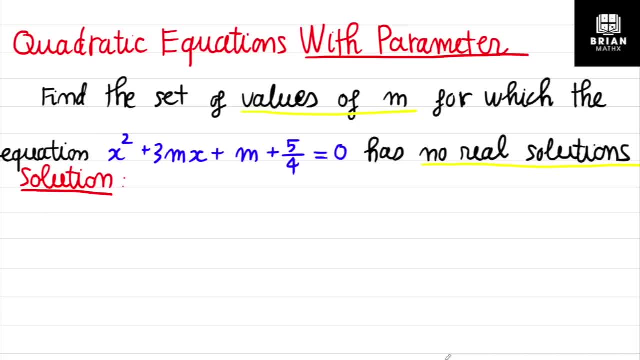 for which the equation here has no real solution. OK, maybe in the last video we learned about the parameter- How can you find the discriminant of a quadratic equation with parameter? But in this video we have to apply that discriminant for finding the value of m. 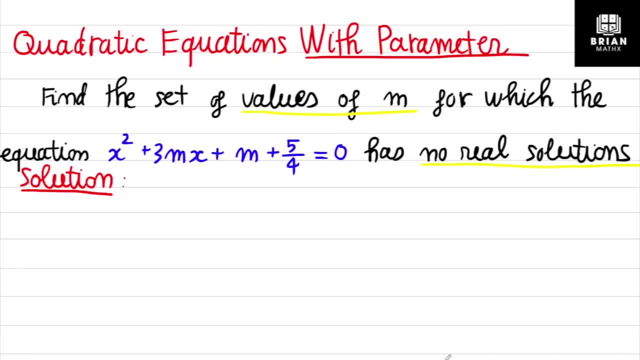 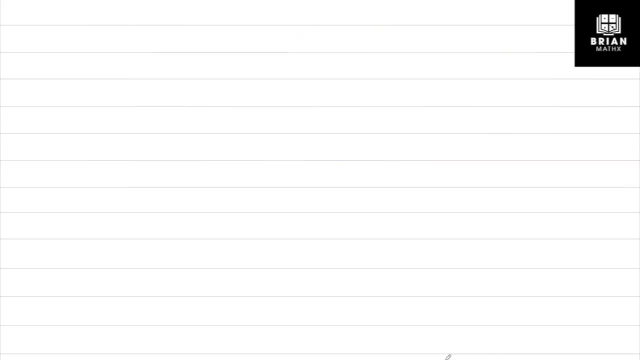 OK, before we working for this question, I need to remind you about the discriminant conditional. So for the discriminant of a quadratic equation you have 3 case. The first case when you have the discriminant greater than 0, it means the quadratic equation will have 2 solutions. 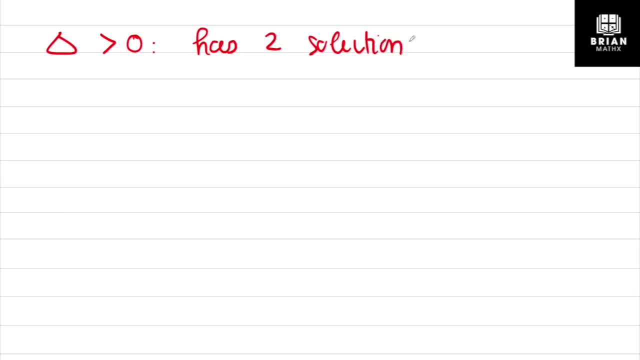 2 distinct solutions or the different solutions, And when you got the discriminant, have value equal to 0, so the equation has 1 real solution, Has 1 real solution or maybe another calling for this one is: oh sorry, this is solution only. 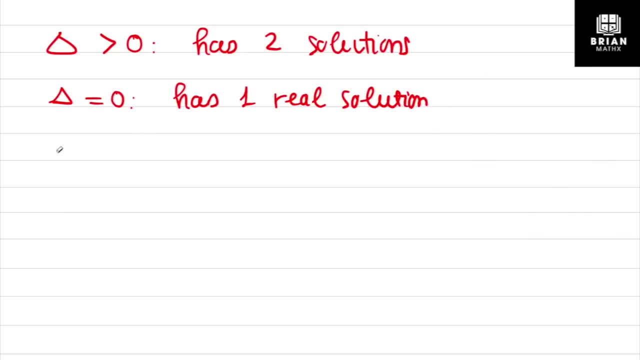 1 repeating solution. And the third case: you got the discriminant less than 0. It means the quadratic equation has no real solution. OK, 0,, 1, 2, greater than equal and less than 0.. 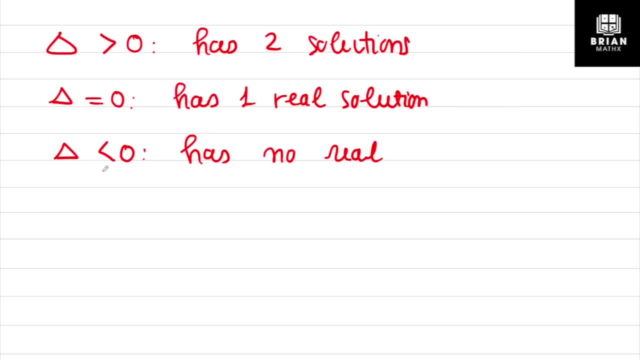 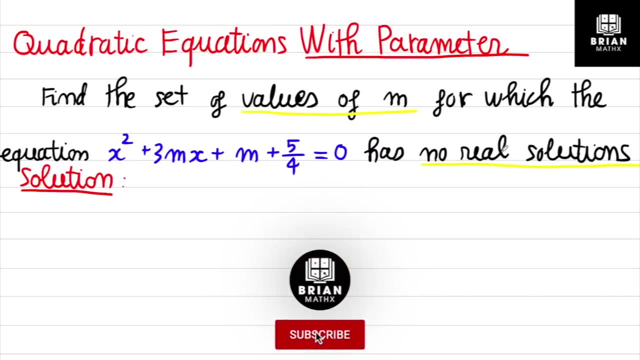 OK, Or positive equal 0 and negative solution here. Yeah, OK, That is the first thing you need to do for solving this equation. And then the blue pen you got here, the x squared plus 3 and x plus m plus 5 over 4 equal to 0.. 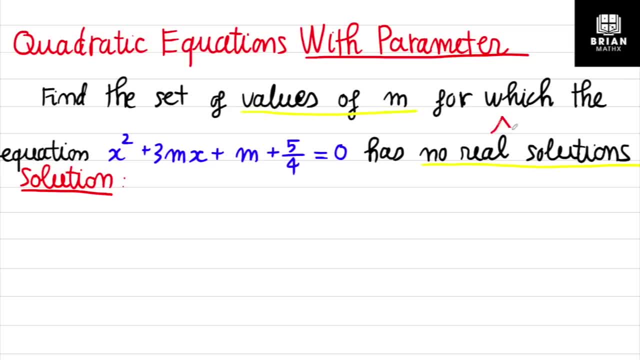 No real solution. What does that mean? The discriminant have to be value for negative. No real solution. And the additional for the quadratic equation has no real solution is the discriminant will be negative value or less than 0.. OK, So, step by step, we will solve this quadratic equation. fighting for m. 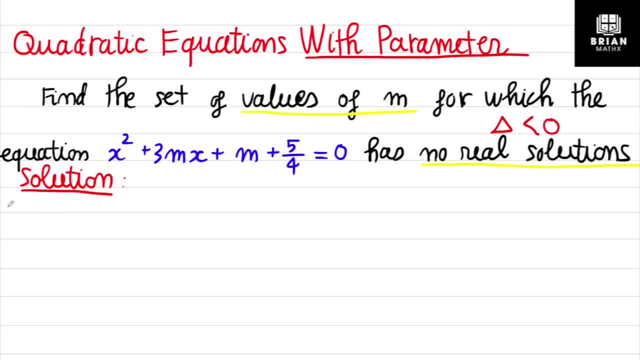 The first thing you need to do is find the discriminant of the blue pen. I mean, you have to determine which is the value of a, b and c. Value of a: equal to 1.. Value of b: you got 3m. 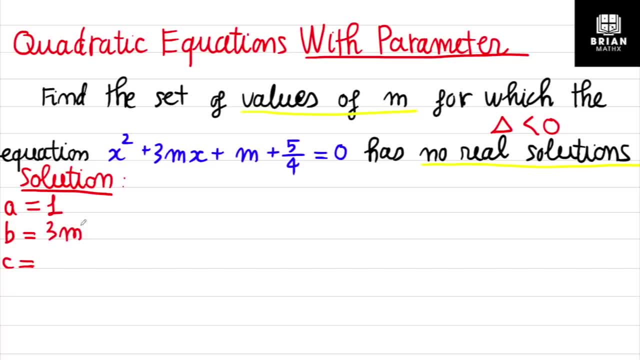 It's not 3, it's not m, It is 3m And the value of c. you got all the number without x equal to constant number, I mean equal to c. So you got c here equal to m plus 5 over 4.. 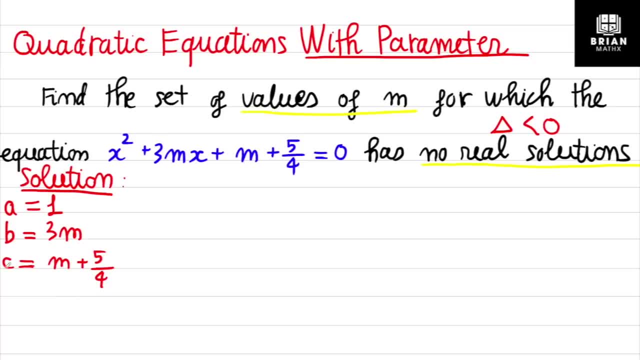 OK, We done for finding the value of a, b, c And the next step we finding the value of discriminant. b squared minus 4ac is 0.. 4ac is the original expression about the discriminant and with substitution for b, a and c: 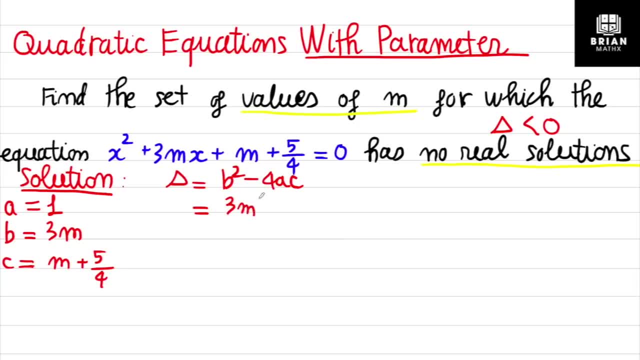 For b. here you got b squared. You should not write down like this, Because the square in this position only 4m. It's not about 3m, So you So want to correct it. you have to put the bracket for 3m. 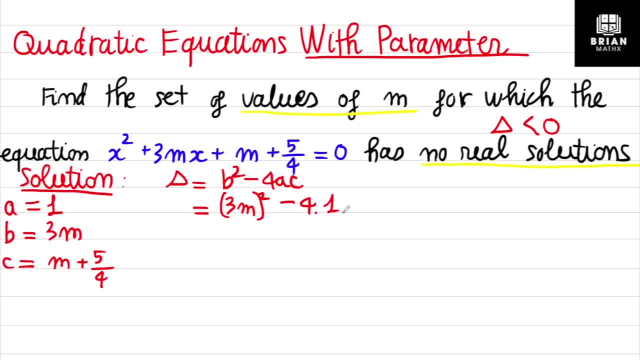 Minus 4ac. OK, So you multiply a and multiply c. Of course you should not write down like this: Put the c inside the bracket like this: OK, And then I will expand here. You got 9m squared minus 4m. 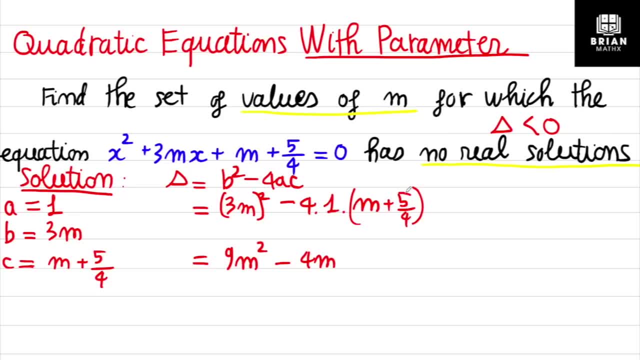 And you expand here, You will got negative 4 multiply 5 over 4.. Negative 4 multiply 5 over 4. And you want to simplify, It's only left Negative 5.. OK, We done for finding the discriminant. 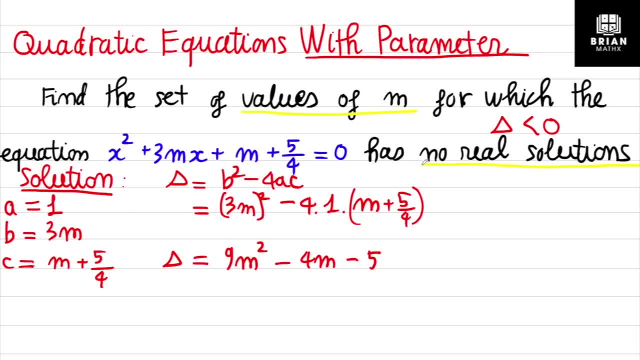 The question ask you about the condition has no real solution. I mean the discriminant has to be less than 0. So this discriminant has to be less than 0. This is the inequality, This is quadratic inequality And I have a privately video about the quadratic inequality you want to re-watch. 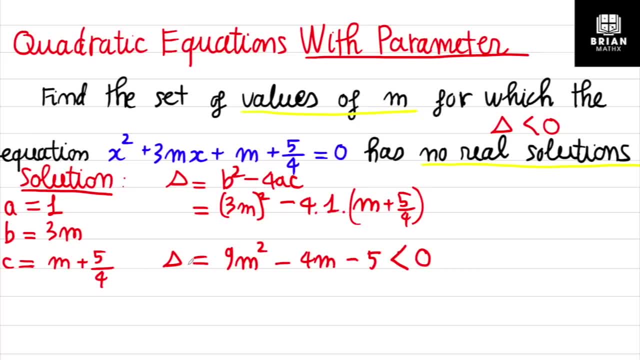 Yeah, The first step for finding the quadratic inequality is You have to find the value for m, For this quadratic equation has to be equal to 0.. So I will finding the value of m first, But finding value of m for this one equal to 0. 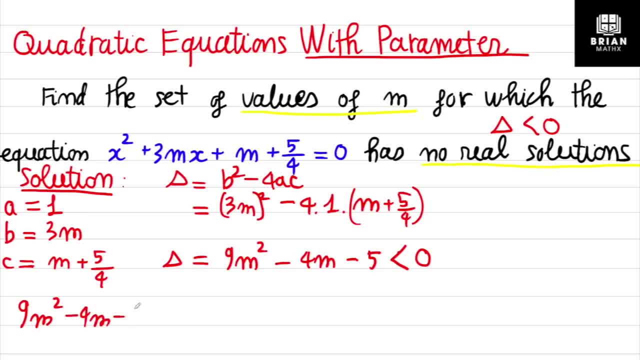 5m squared minus 5m negative 5, equal to 0.. You got a true value of m. The first. you got m equal to 1.. And true, you got m equal to negative 5.. Negative 5 over 9.. 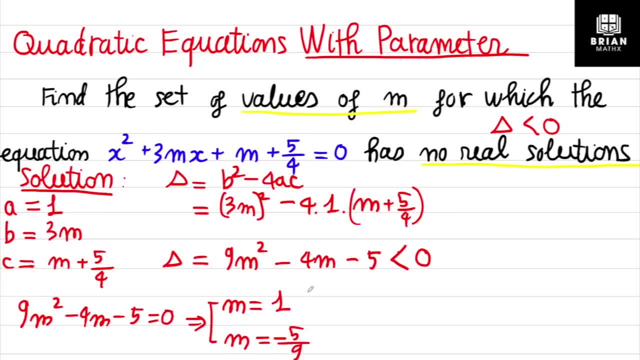 OK, You can using your calculator And after that you finding the number line. The number line for this question will be here: Negative 5 over 9.. And here is 1.. The larger number will lies on the right hand side. 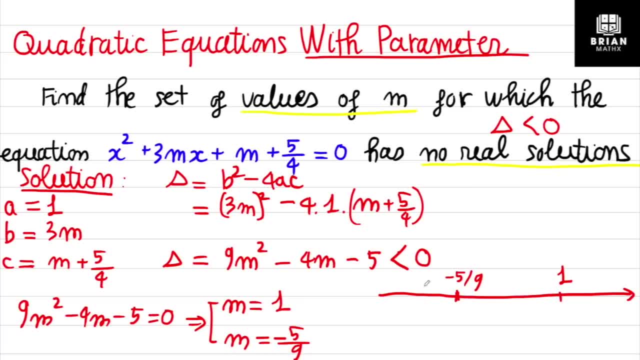 And the smaller number will lie on left hand side And the true value of this number, True value of m, will divide This number line for m into 3 parts: This one, The middle one And the right hand side one, And I want to find the positive or negative part. 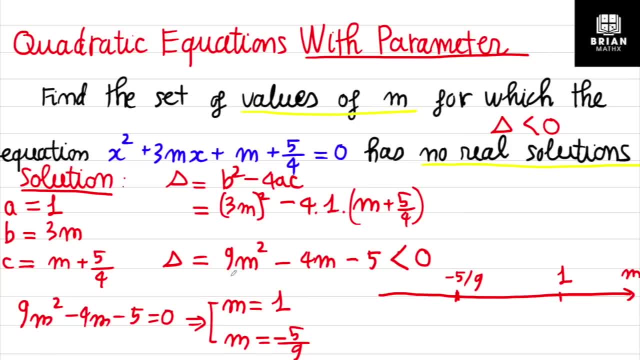 I mean I have to determine the value of a, But it's not a. here You have to finding the value of a for quadratic equation In quadratic inequality. I mean here Because we got here a equal to 9.. It's not 1.. 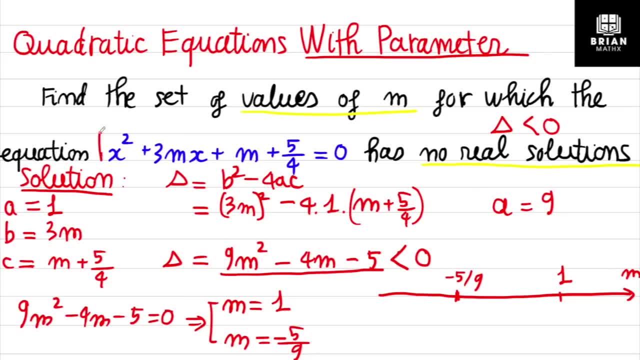 Because 1 here is value of a for this quadratic equation, But for quadratic inequality I have to find value of a for quadratic here, For quadratic here, So a equal to 9. It is positive And the true part outside the number line here will be positive. 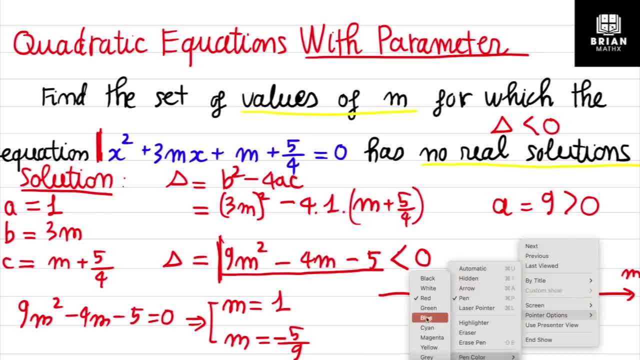 I will change the number here, I will change the point. So this one will be positive, And here is positive, And the negative part? The negative will appear in the middle part. So the question asks you about the less than 0.. 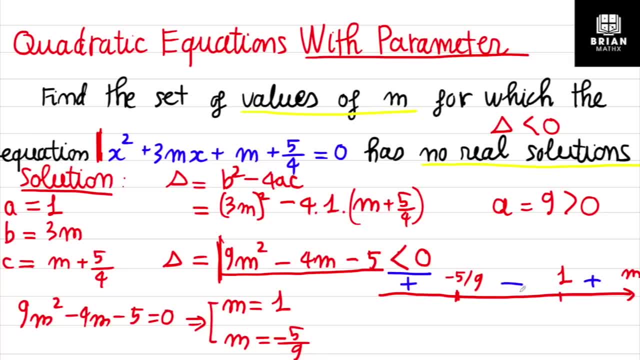 So negative. I want to find the negative part. Which one? Yes, Middle part. So middle part is right hand side of negative 5 over 9.. And left hand side of 1. So you will have the value.